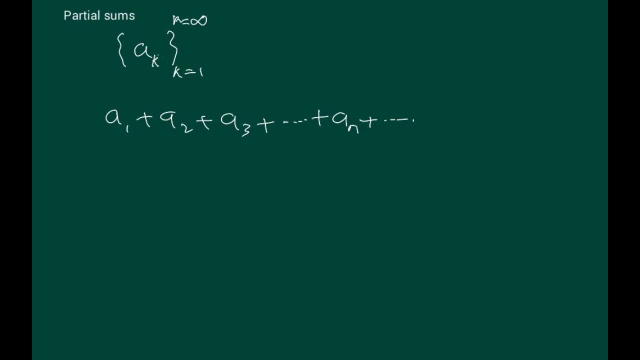 plus a AN, plus so on and so forth. Now, if we think about this as basically defining a sum, S1 as the first term, A1 and let's say S2. okay, let's say S2 is the sum of the first two terms. so it's. 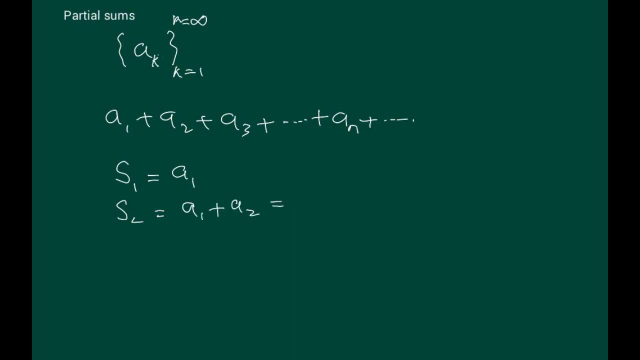 A1 plus A2, which is really the same as S1 plus A2.. So then S3 would be, of course, A1 plus A2 plus A3. sum to the three terms, the first three terms, which is essentially just really, if you think about it, it's just S2, okay, plus A3, and in the same way we can go down this list and get to. 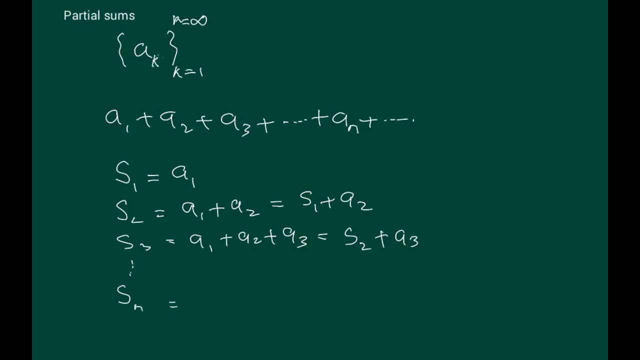 Sn, which appears to be, of course. well, officially it's, or formally it's just this sum, But using this idea, we can write it as Sn minus 1 plus An. So basically it's a sum to the n minus 1th term. okay, which. 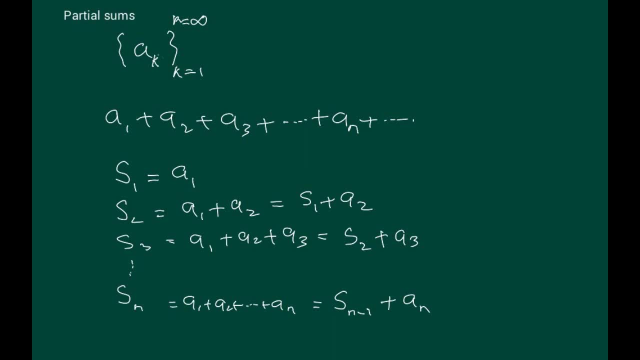 is this S minus 1 and the next term. okay, Now, these S's basically are a sequence, We can think of them as a sequence of terms And therefore, so we can say that we have a sequence here: S1, S2, S3, Sn and so on up to infinity. Now, if we can show that this sequence, 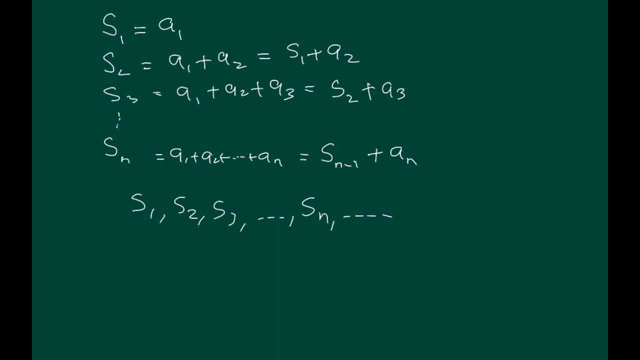 which is the. these are all partial sums, These are basically these S's are the partial sums. So if these partial sums, the sequence of partial sums, is convergent, then we can, we will. it would mean that the series of which these partial sums or to which these partial 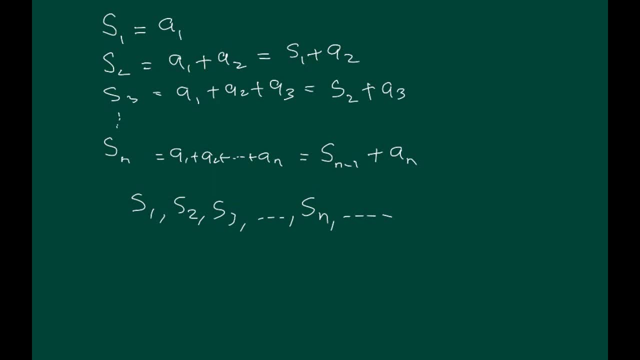 sums belong is in fact converging to that sum. So if this is a convergent series and suppose it converges to that sum, then we can say that the sequence of these partial sums converges to. okay, if it were to do that, I mean, what would converge? what I'm 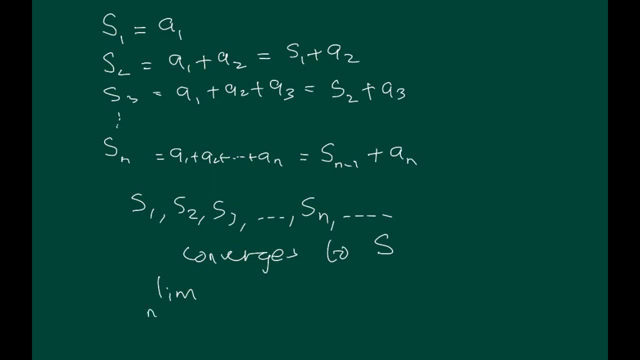 saying is that if we were to test this as a sequence, we've just done sequences, so Sn, essentially okay, is what I'm talking about, and if this is equal to S, then this S, obviously it's a convergent sequence. but what is this S representing? It represents: 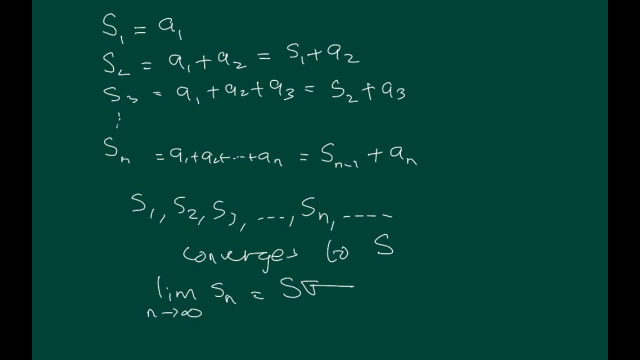 the partial sum, It represents, in fact, the entire entire series. okay, It represents the entire series and what we can say is that if this, if it's converging to this sum, that means the series is converging to that sum. So, in other words, in other 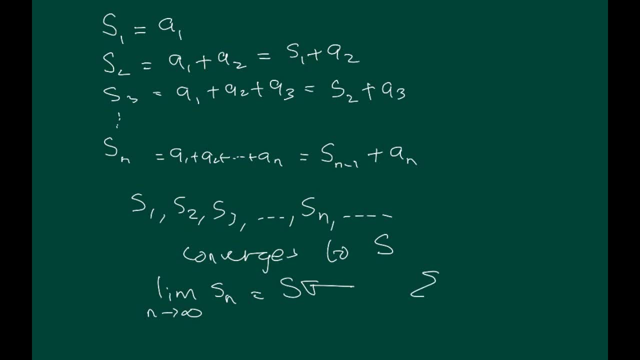 words, what we started with would be the series k equals one to infinity and it's- and of course it's- a convergent series. So let's look at a particular series, how we would study it under this sort of criteria. 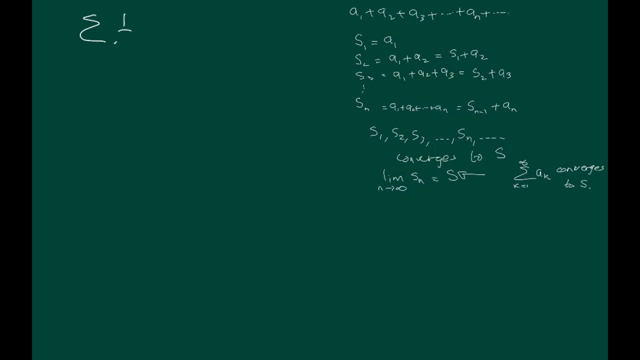 Okay, One over two to the power. k. k equals one to infinity. Let's see what we can say about this particular series. So if we were to break this up into the, into the same concept as a partial sum, then the way we had it was that the nth term, or if we start with the, 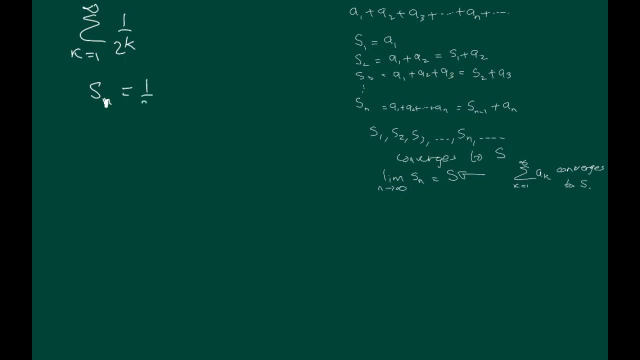 first term, say S1,. S1 is going to be one over two, S2 is going to be one over two plus one over four. Okay, which is three-fourths. S3 is in fact three over four plus one over two, cubed which? 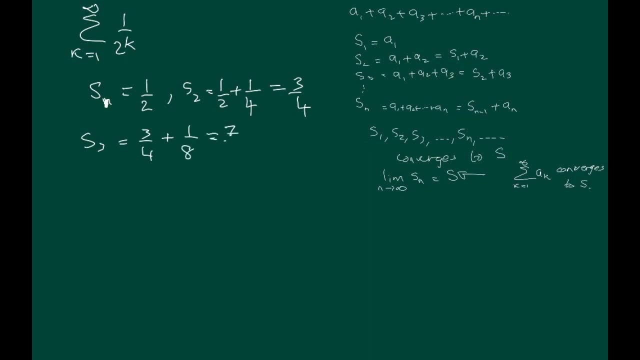 is eight, so it's equal to seven-eighths, and so on S4, S4 is going to be seven-eighths plus one over two to the four, which is one-sixteenth, So it's equal to fifteen over sixteen. Now it's interesting. it's interesting that if 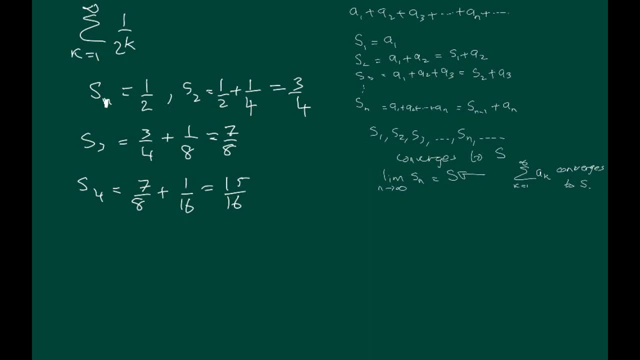 you notice, we can break this up as follows: The S1 is basically one minus one over two. S2 is one minus one over two squared. S3 is in fact one minus one over two cubed, which means I have my S1..